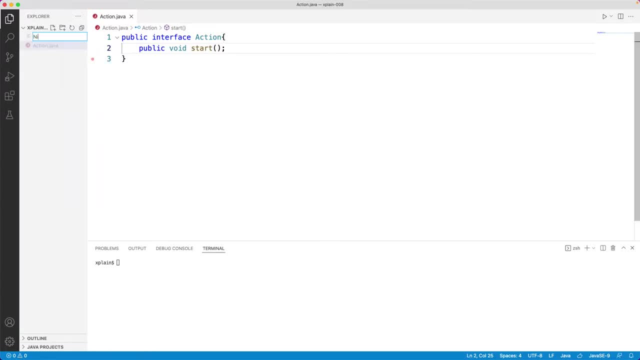 create a new class called nissanjava and this will have this: will first implement, implements action and add override public void, start in that we would like to print line and it's going to say lego, an action, implements action, starting nissan, and the third class would be: 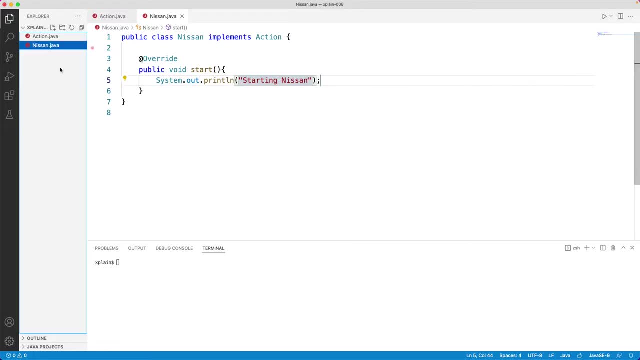 hondajava. and the third class would be hondajava- hondajava that will implement action same as nissan. same as nissan action, Nissan Act Override Public Void, Start And Systemoutprintln Starting Honda. Now we would like to create abstract class called Vehiclejava. This is an abstract class, So we will call this public abstract class Vehicle. 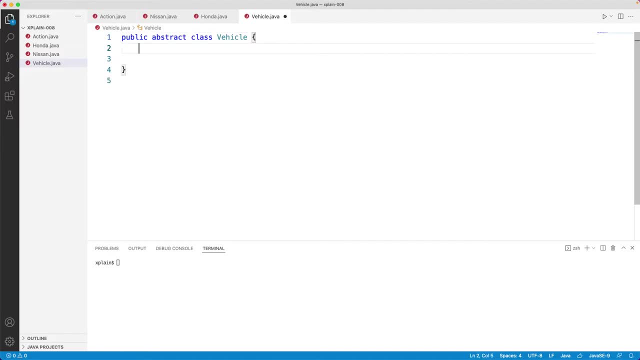 Within that, we would create a protected action, Because we would like to use this action in other classes Action. Then we will have a protected constructor Vehicle With action as parameters, And within this we would like to set action equals action. 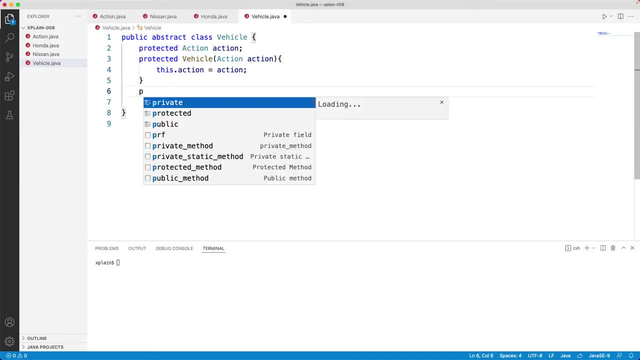 And, at last, we would like to create an abstract method, Public Abstract Void Start. This would be the same method as the interface. Once the Vehicle class is created, let's go ahead and create a concrete class called Carjava. 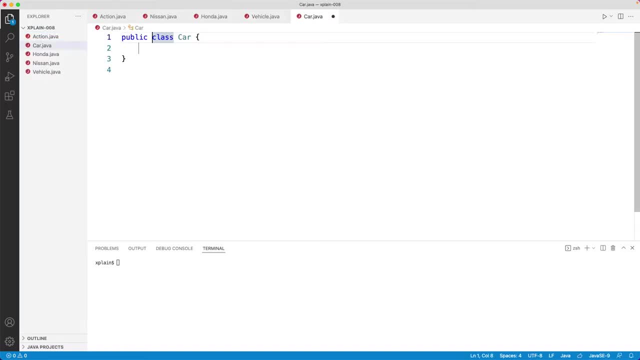 That'll extend our abstract class Vehicle. Within this we will create a constructor Car That would take action. Action Within that we would like to call Superjava constructor, that is, vehicles constructor. and that is done. let's override start method and call. 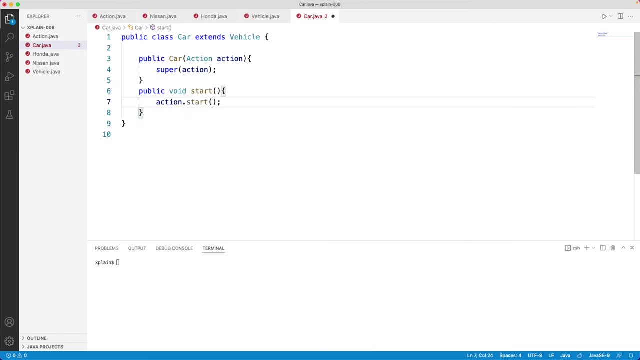 action dot start now. we have created a concrete class. now the final class would be bridge test dot Java. that will have our public static void, main, public topic, why main string args. and then within this, we would like to create vehicle Nissan equals new car, new Nissan and using the 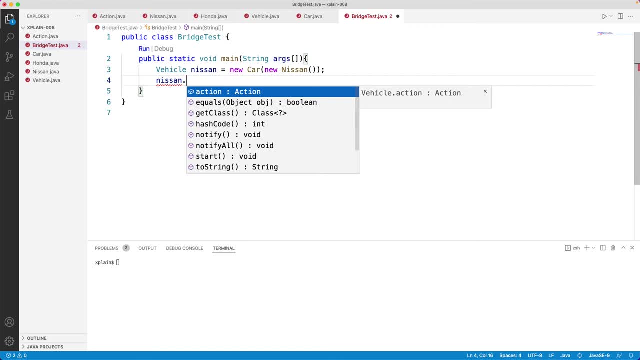 Nissan and using the object, we would like to start Nissan vehicle and again we would like to instantiate vehicle. Honda equals new car, the action that we pass this Honda and finally we would say Honda dot start here. we have instantiated both Nissan and Honda and we are starting both the